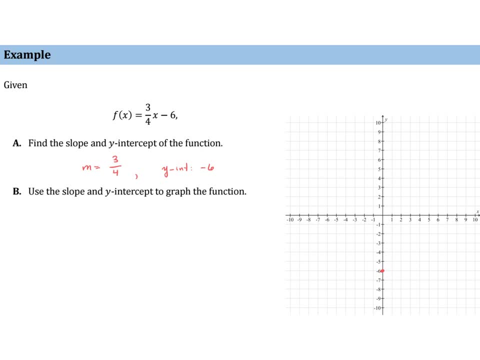 So we will go up 3, to the right, 4.. Now we connect those two points. If you wanted more points, you could go up 3.. You could go up 3 and to the right, 4 again. or we could go down 3 and to the left 4.. 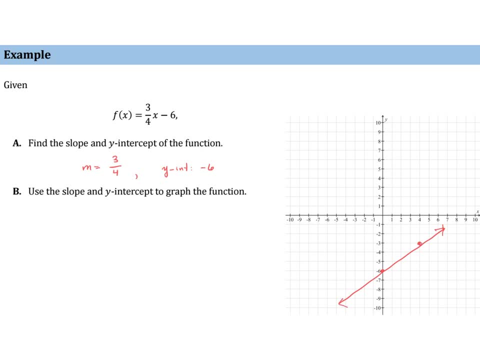 And so there is our line. Now let's look at another one. This time we have g of x equals 5. So the best way to think about this is: if we have g of x equals something times x plus b. 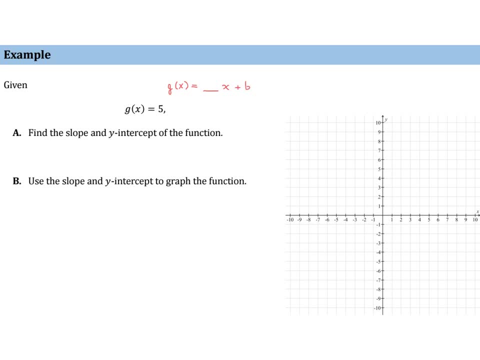 what could go in for this coefficient of x, so that the x-term would disappear And the answer, of course, would be 0.. So g of x equals 0x plus 5, means the slope is 0, and the y-intercept is 5.. 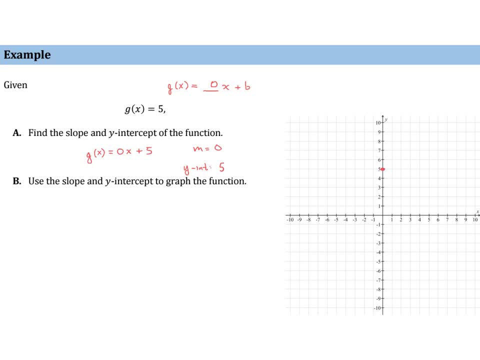 So y-intercept is 0, and the y-intercept is 5.. And then a slope of 0 means that we will have a horizontal line. Now in our third example, our slope is negative 2 thirds and our y-intercept is 7.. 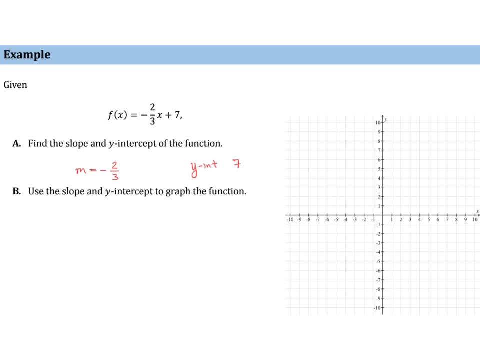 And our y-intercept is 7.. And our y-intercept is 7.. So now, what's it mean to have a negative slope? So now, what's it mean to have a negative slope? Well, if I have negative 2 thirds. 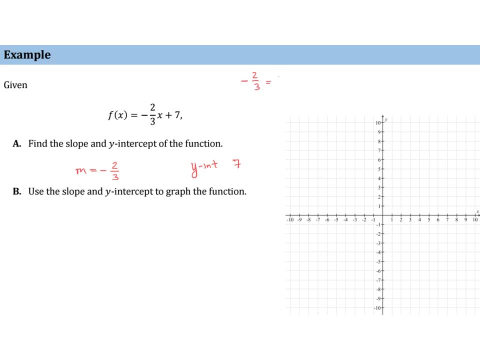 that is because I've divided two numbers and one of them is negative. So I could have negative 2, divide by positive 3.. So if we start off at 0, 7, I could go down 2, to the right 3.. 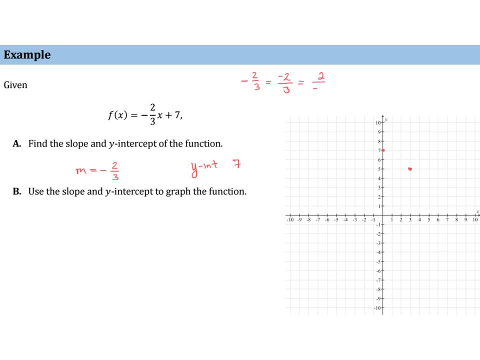 Or it would also work if the negative were in the denominator. So 2 divided by negative 3, likewise would give us a negative 3.. would give us a negative 2 thirds. So that would mean I would go up 2, to the left, 3.. 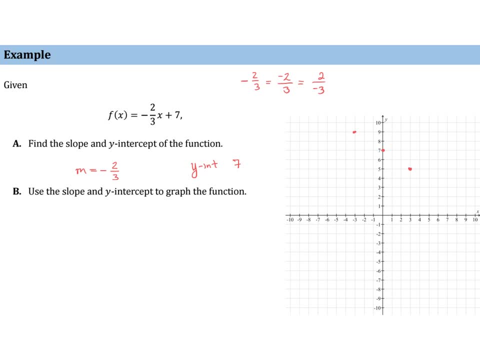 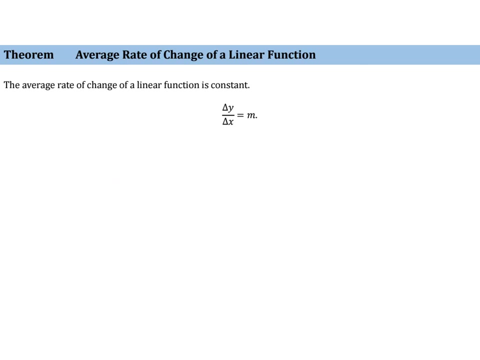 And either way, we end up with the same line. Now, what is slope? The average rate of change of a linear function. The average rate of change of a linear function is the slope of our line. is the slope of our line And as long as it's a linear function, 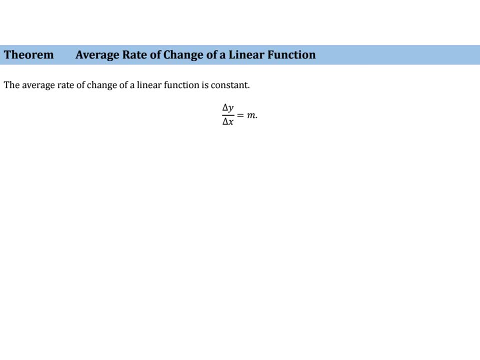 that average rate of change is constant. So no matter what two points you choose on the line, So no matter what two points you choose on the line, the rate of change between those two points is always the same, is always the same. So how do we know this? 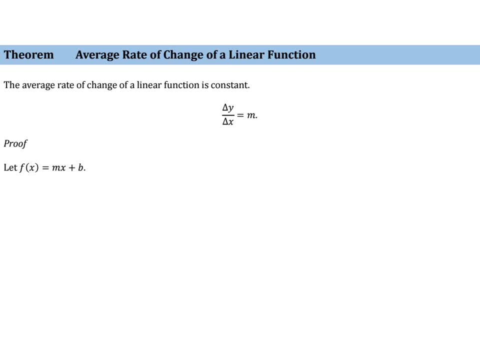 Well, the average rate of change? Well, the average rate of change is given by the difference quotient. So if we start off with a linear function, f of x equals mx plus b. let's look at the difference quotient. So delta y over delta x is. 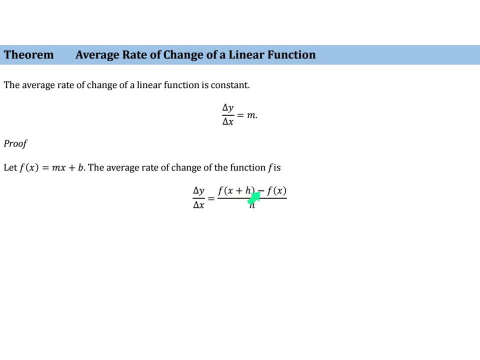 given by that difference quotient: f of x plus h minus f of x over h, f of x plus h minus f of x over h. So we will take x plus h and put it in for x and put it in for x, So f of x plus h. 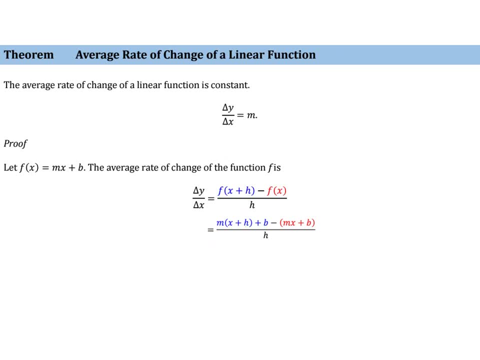 is m times x plus h plus b, is m times x plus h plus b. Then we'll subtract off f of x, which is mx plus b, and we'll divide by h and we'll divide by h. Well, if we distribute to m, 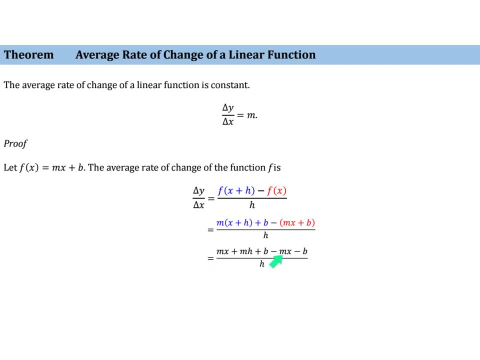 we get mx plus, mh plus, b minus, and then we'll distribute: so minus mx minus b. Notice: mx minus, mx disappears, b minus b. also add to zero. So we are left with mh over h, mh over h, which is just m. So 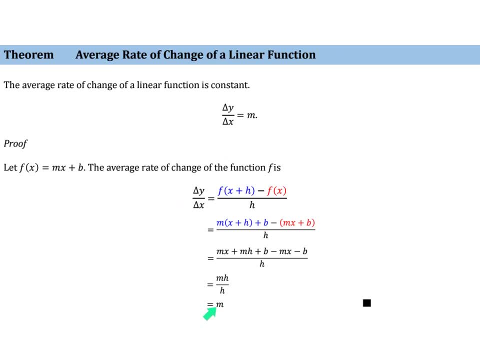 the average rate of change is always the slope of the function. This is not all that exciting And don't worry about ever having to really worry about this proof, But the application of it is this: We can determine whether or not a data set is linear by looking at. 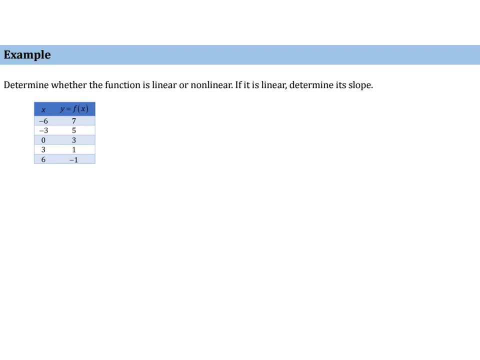 every point in the data set and simply seeing if the slope between the two points is constant. So if we look at the change between each one of these x values, notice delta x is always 3.. We're just adding 3 between each one of those. 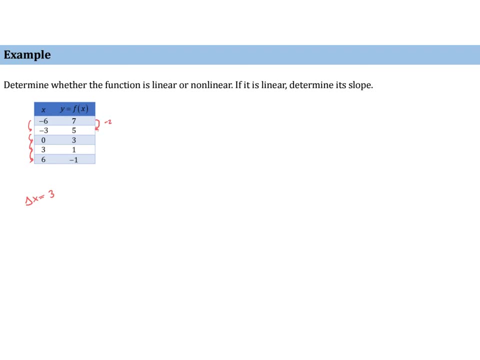 But what about here? Here we are subtracting 2, then we're subtracting 2, then we're subtracting 2, then we're subtracting 2.. So here the delta y is constant. It's negative 2.. 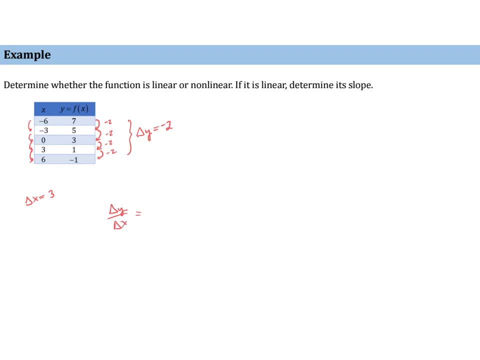 So delta y over delta x equals negative 2 over 3. Negative 2 thirds. That means that this is indeed a linear function. What about in this example? Look at your change in x. We're adding 5.. Adding 5.. 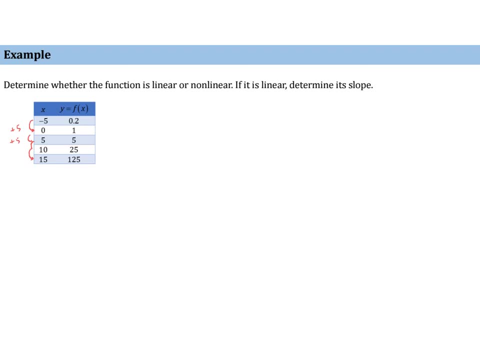 And that's consistent throughout. So delta x is an addition of 5.. What about here Delta y? here is 0.8.. Delta y here is 4.. Then 20.. Then 100.. So delta y is not constant. for that constant delta x. 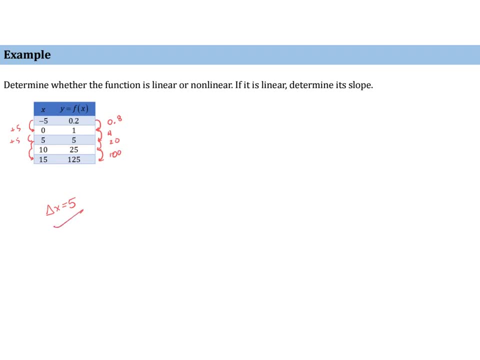 So this is non-linear, So we're subtracting 2.. Now how can we interpret slope in relation to the graph? Well, if the slope is positive, then the linear function is increasing And we would see a line that goes up. 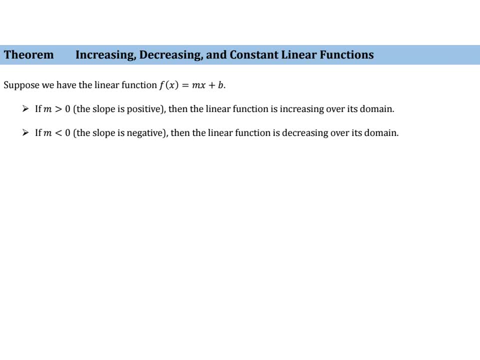 If the slope is negative, then the function is decreasing. So left to right, the function would fall. The line would fall If m equals 0, then the function would fall. So the graph is a horizontal line If you look back. 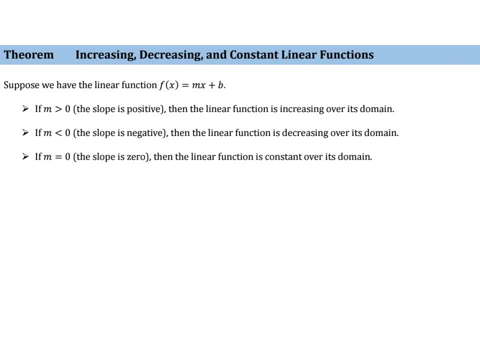 at the examples from this video, you will see that we've seen a line with a positive slope, a line with a negative slope and a line with a zero slope, And you will be able to see that the graph increases or decreases based upon.